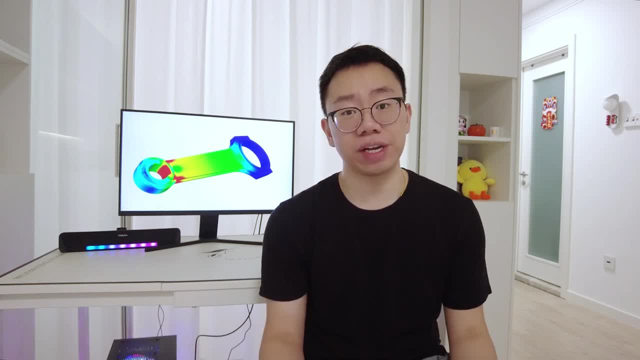 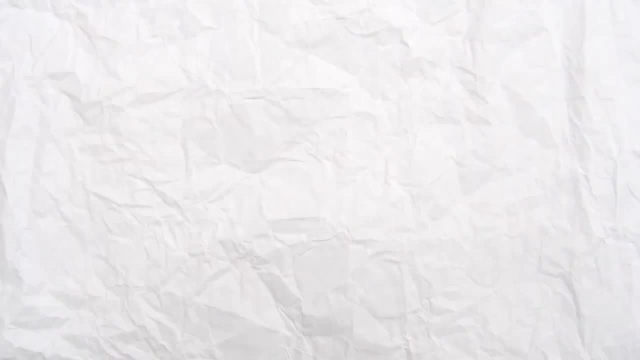 you should know before getting into engineering, based on my experience, so you don't end up having any regrets or discover any unpleasant surprises along the way. You might be studying engineering for the money, or you think it's the best major for job security. Maybe your parents are forcing. 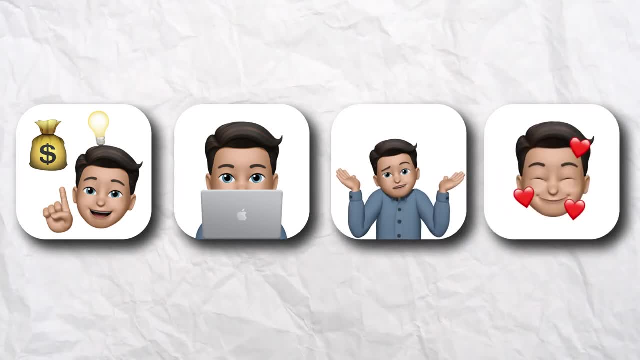 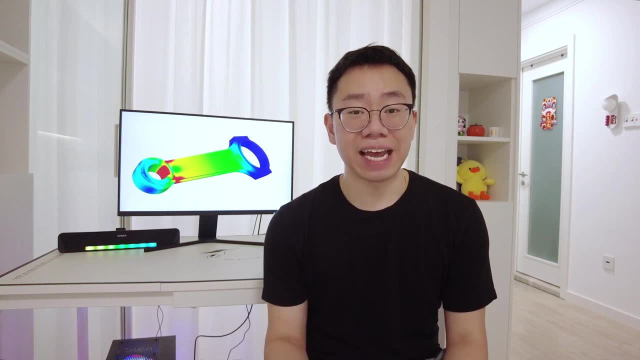 you to, or you truly love, or you think you love engineering. These are all totally different things that you might be feeling about your career in other countries. I don't know if you legitimate reasons. I chose engineering for many of the same reasons, but at the end of the day I 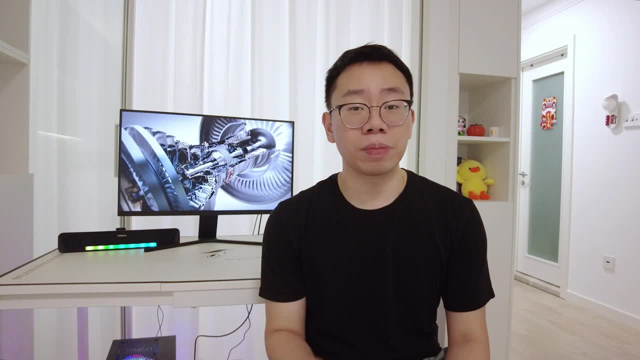 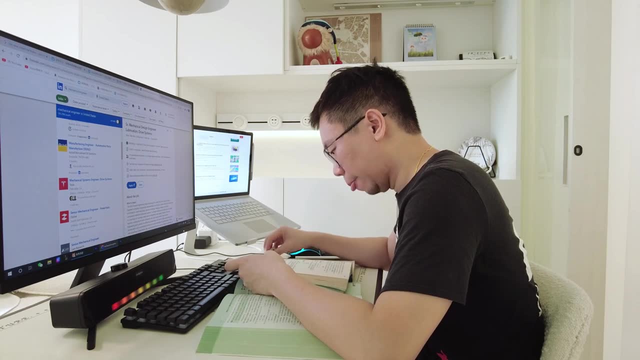 wish somebody told me the things I'm about to tell you, because it would have made my life a whole lot more enjoyable and a hell of a lot easier in terms of studying, job hunting and stepping foot in industry. The first thing you should know is engineering is one of the hardest majors and 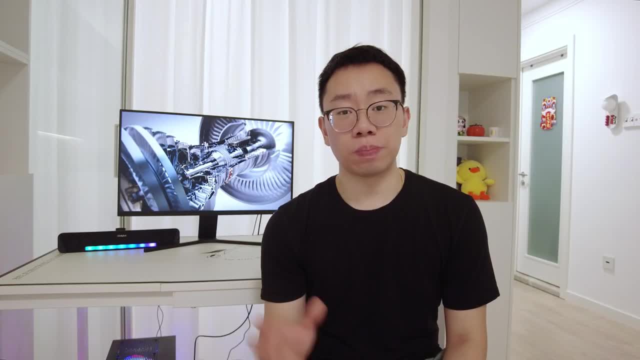 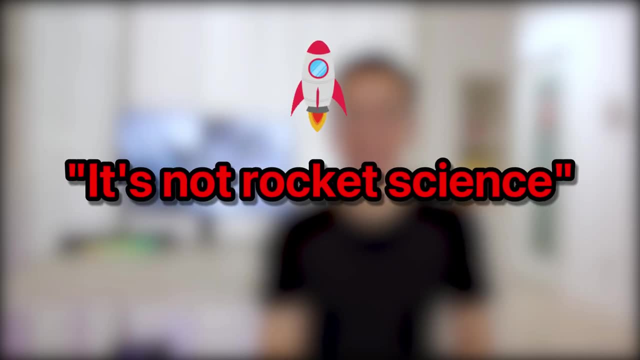 definitely won't be a walk in the park, so be mentally prepared. Before getting into engineering, I knew it was going to be hard, but I didn't know it was going to be this hard. The idiom it's not rocket science suddenly makes so much more sense now. I studied mechanical engineering, which is 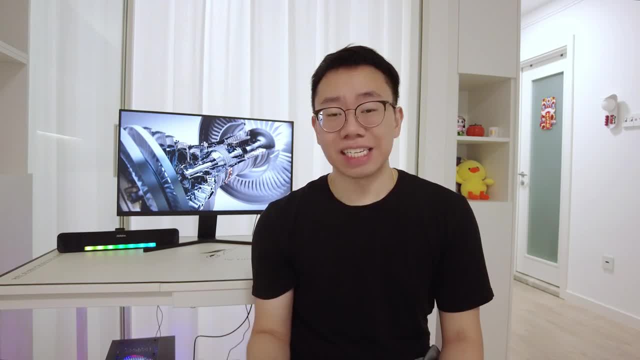 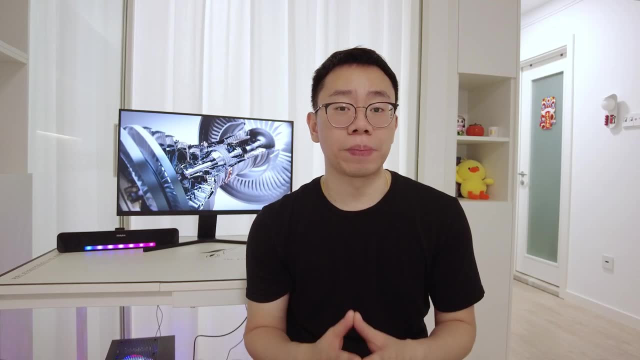 probably one of the broadest engineering disciplines. My first and second years were the most challenging for me because I wasn't used to learning the massive amounts of material taught in class in such a short period of time and the pace at which everything was taught was lightning. 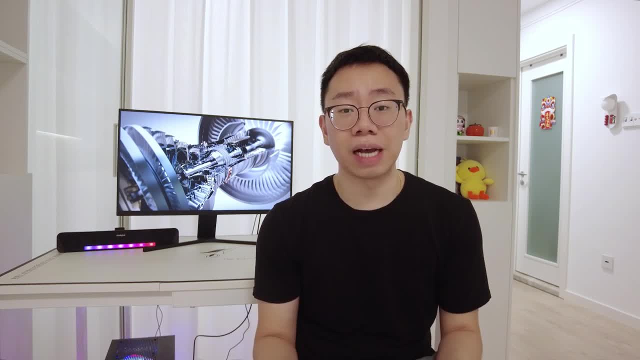 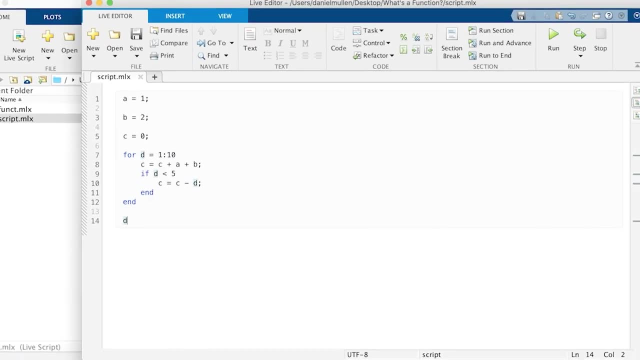 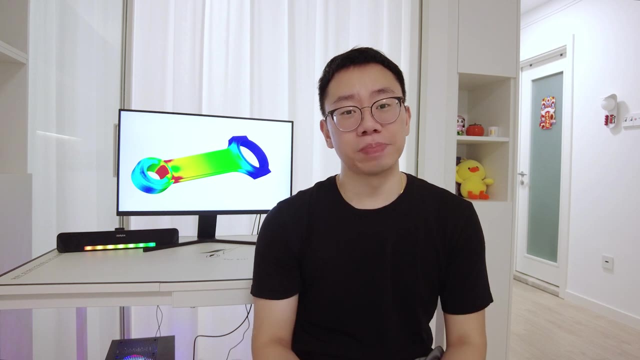 fast. It also took me a while to develop an engineering mindset for problem solving. In the first semester of university I took a mandatory course called Intro to Engineering Computation. that taught us how to write scripts and solve engineering problems using MATLAB. I remember freaking out right after taking the first midterm and calling my mom to tell her. 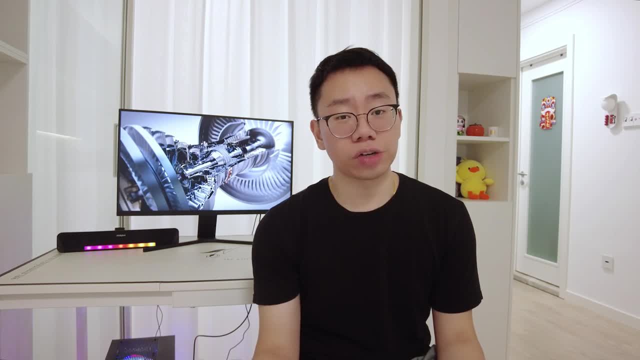 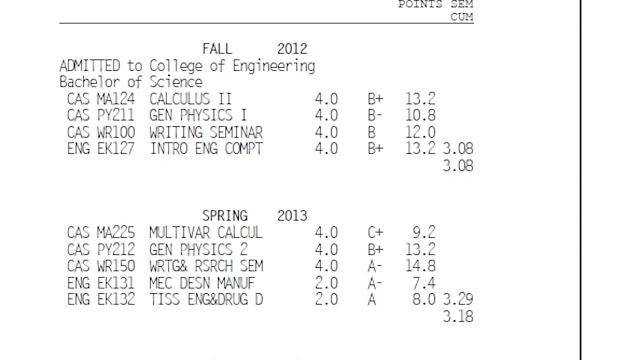 that I bombed my exam and that I was going to fail the class, lose my scholarship and drop out of school. As crazy as it sounds, even though I got a 70% on the first midterm, I still ended up getting a B plus in that class and everything turned out just fine. I realized that I 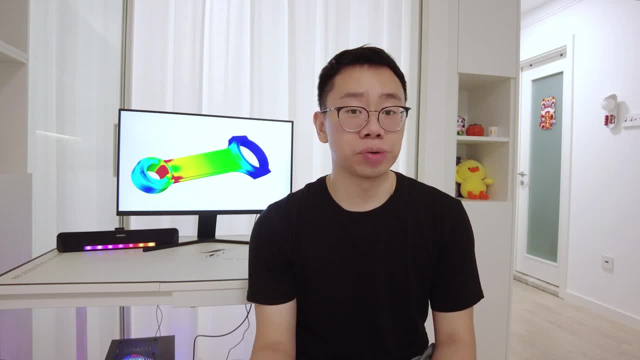 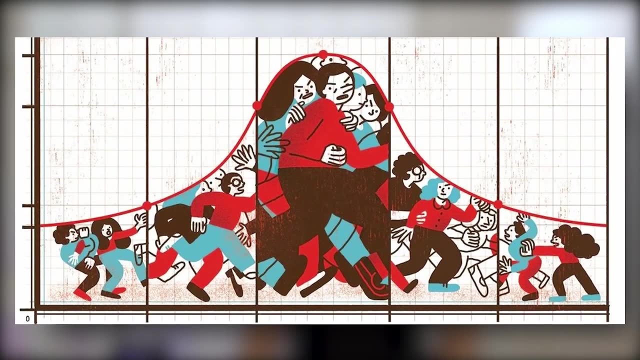 failed the exam to be hard. it's likely that other students will too, and the final grade that you get is all relative to other students in the class. 10 times out of 10, the professor will apply a curve. so if you feel like you did bad on the exam, don't stress out too much until the exam and class. 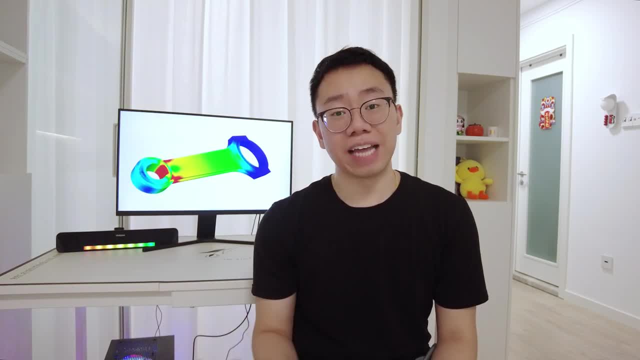 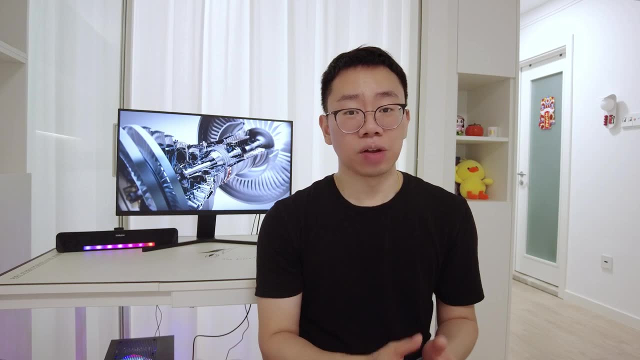 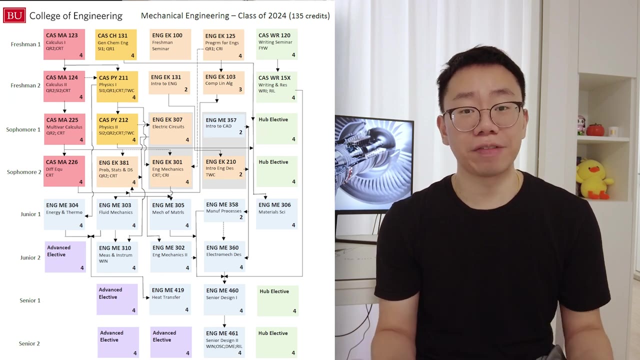 averages actually come out. It's definitely normal to have doubts and feel stressed out throughout your engineering journey, but try not to worry too much about the result and focus instead on learning the material to the best of your abilities. Now one of the biggest problems regarding the mechanical engineering curriculum that I face. 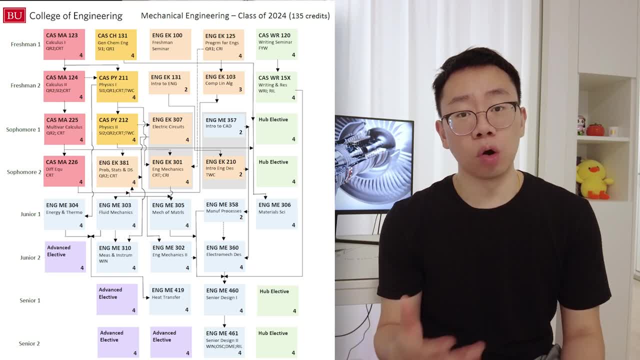 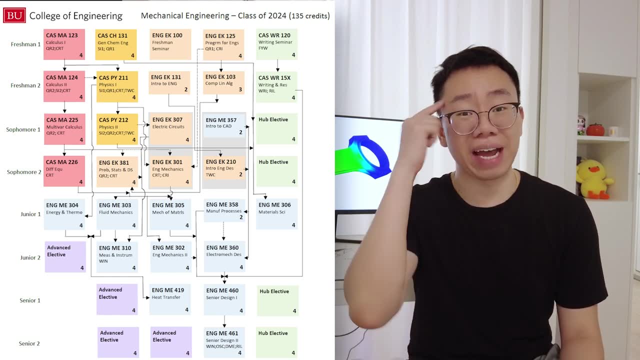 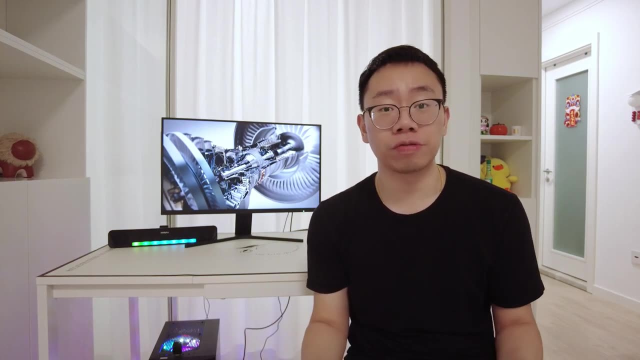 is figuring out which core engineering courses are the most important for my career and organizing all of the key concepts and retaining all that information in my head for exams and interviews. I'm sure many of you will encounter the same issue, so I decided to do you a huge favor. I went back. 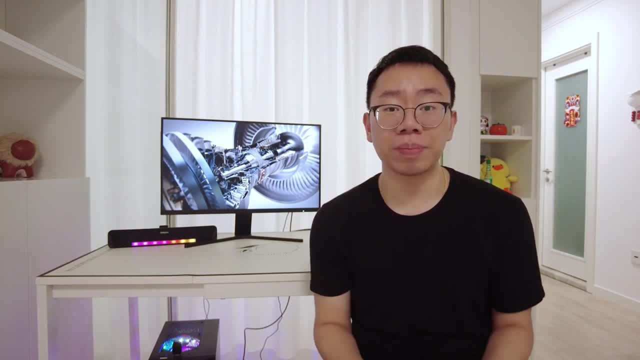 and summarized all my notes that I took in university for all the mechanical engineering classes that I think are important. I'm going to talk a little bit more about mechanical engineering courses that I think are important and created a detailed one-page cheat sheet for each class. 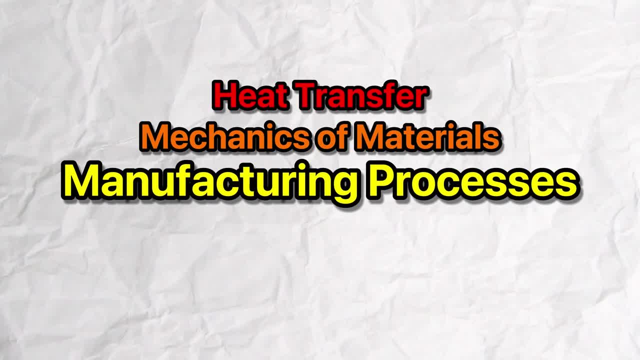 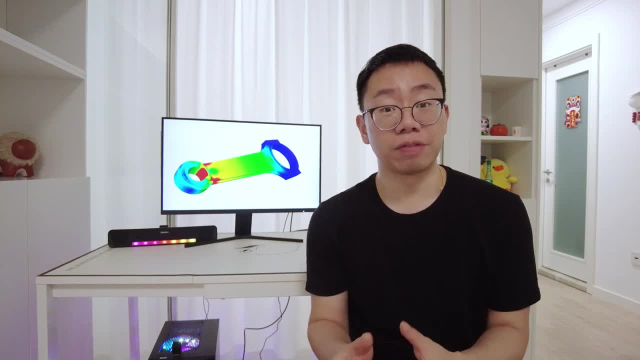 including heat transfer, mechanics of materials, manufacturing processes, fluid mechanics, product design and a whole bunch more. With these cheat sheets, you can review them before your interview or exam and know exactly which concepts to focus on. Now, I'm not saying you don't have to read the 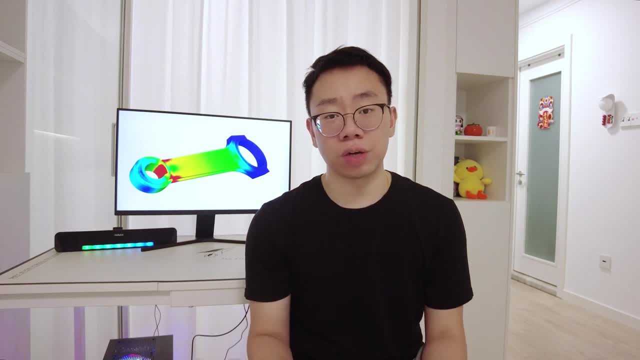 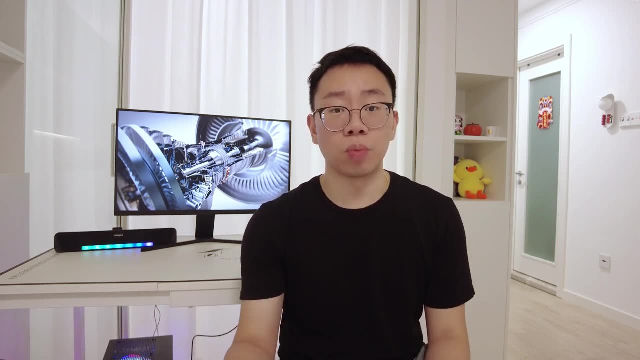 textbook anymore or that you can skip class. You'll still have to put in the work, but these cheat sheets will really help you to retain the key concepts taught in these classes and will help you learn the material more efficiently. So if you're interested, link in the description. 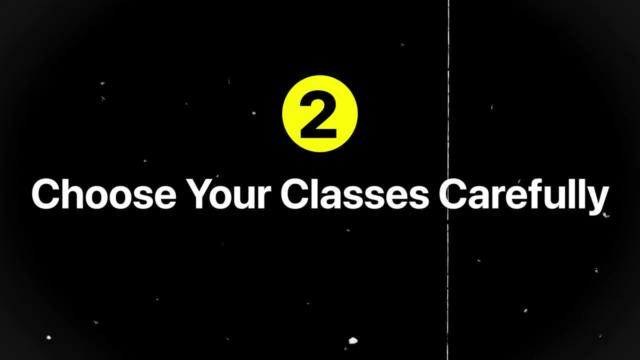 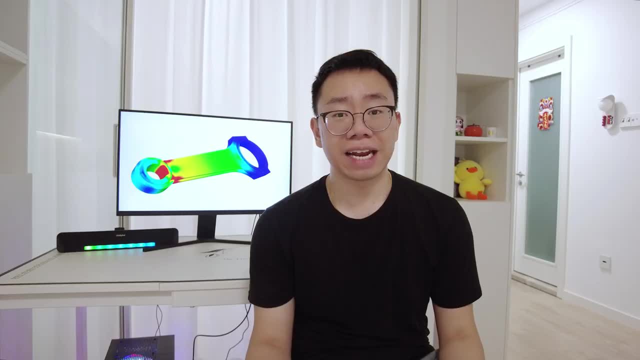 below. The second thing you need to know is choose your classes carefully. What do I mean by this? Well, I attended Boston University, which is considered a pretty big private university, and every semester, multiple sections of the same course, taught by different professors, were offered. 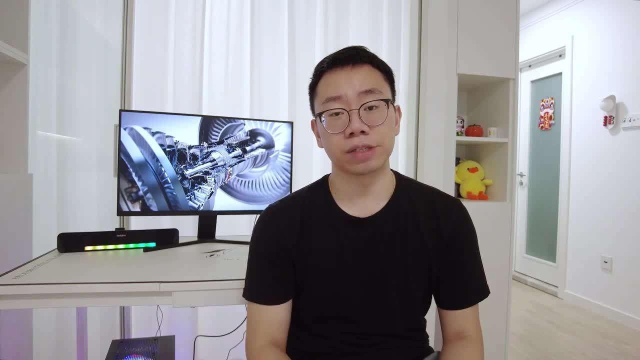 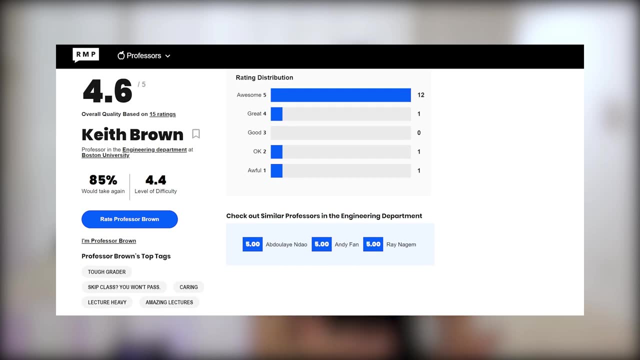 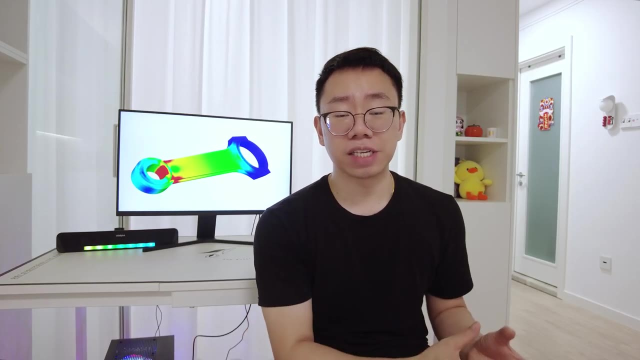 Let's assume your school requires you to take fluid mechanics. What you should do is find out which professors are teaching fluid mechanics that term. stalk them on RateMyProfessorscom to see what other students are saying about their teaching style, class format and grading system, and pick a section that works best for you If you know you. 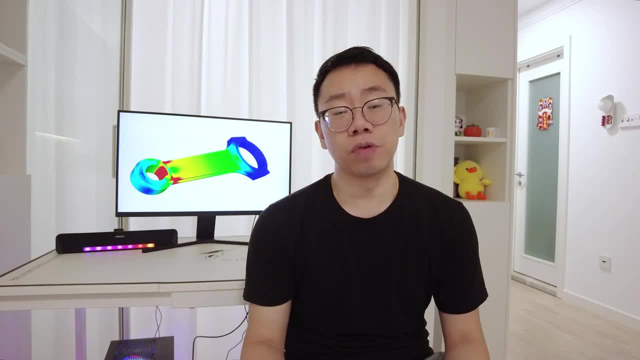 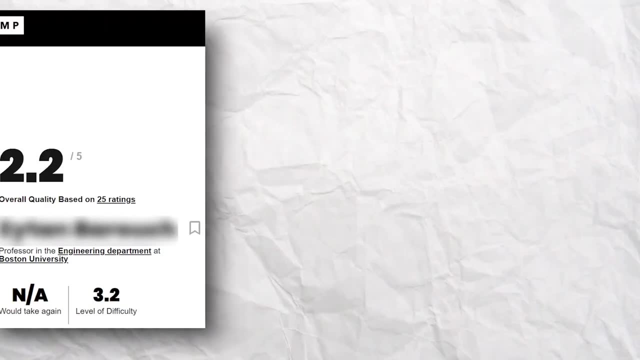 aren't a morning person, do yourself a huge favor and avoid choosing an 8 am section. I made the mistake of enrolling in a material science class taught by a professor with two and a half out of five stars on RateMyProfessors. Another professor with four and a half out of five stars was also. 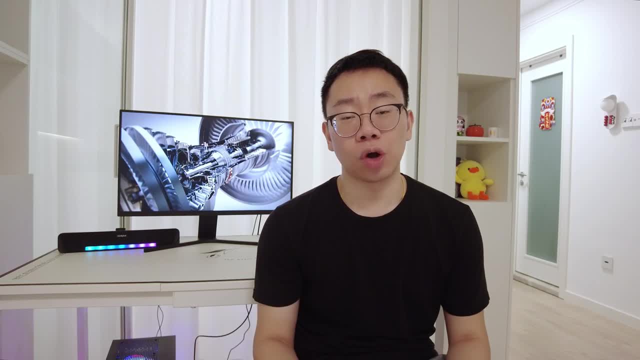 teaching the same course that semester. If you're interested in learning more about fluid mechanics, please refer to my excel course link in the description box. But when I found out it was already too late to switch. A professor can really make or break your 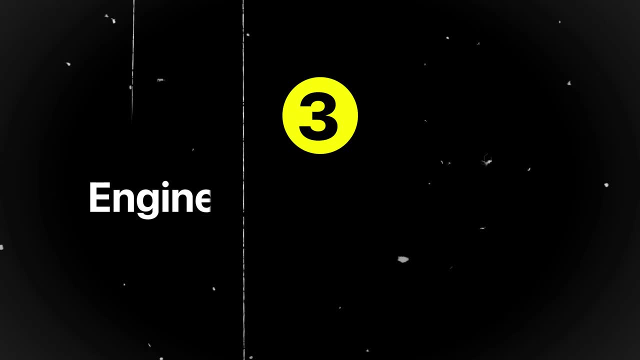 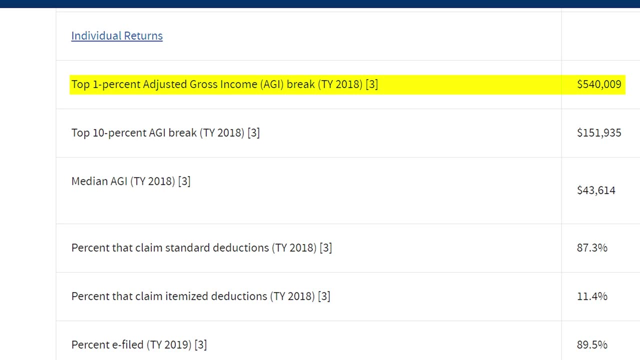 grades, so do your due diligence. You should also know that engineering alone won't make you rich. I've defined rich as making at least 500 thousand dollars a year in the United States, which puts you in the top one percent. As an engineer, you'll make a salary needed to live a 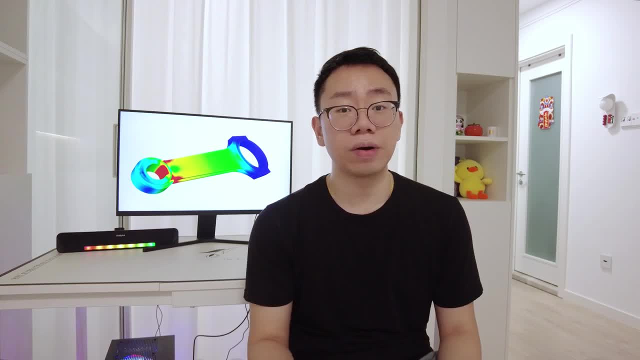 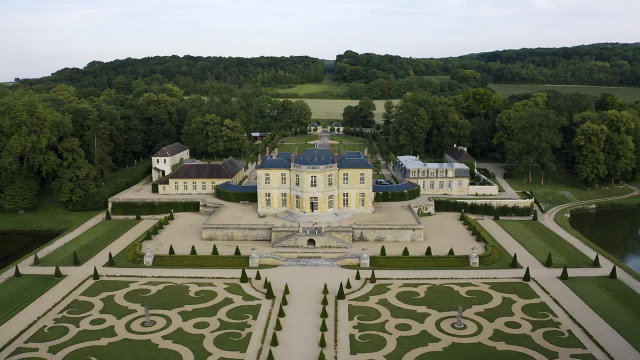 very comfortable middle-class lifestyle, which includes eating out, buying a nice car and house, going on vacations and saving up for your contract for college and living in the city. Do you know any other on vacations and saving up for retirement? However, you won't be living in a mansion or 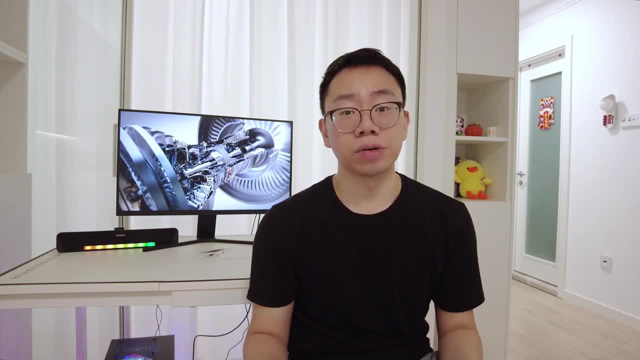 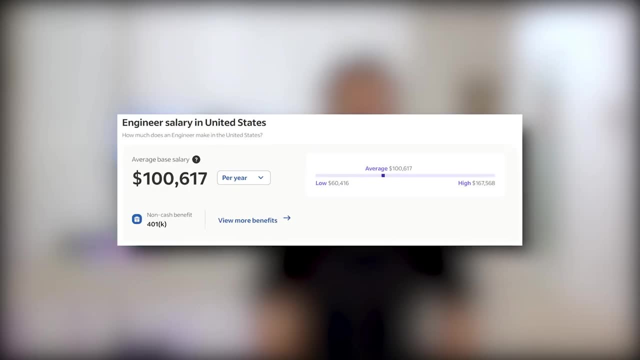 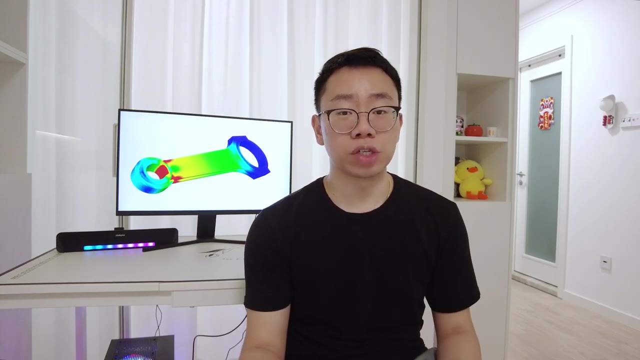 owning a private jet, unless you have several other good side hustles that are generating extra income. Depending on what type of engineer you are and where you work, you can expect to make anywhere between $60,000 to $167,000 per year. There are also many engineers who become rich. 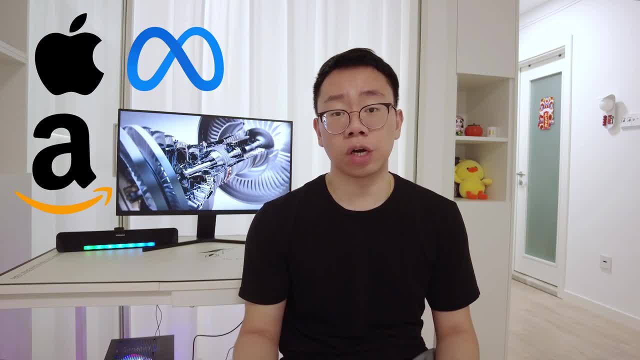 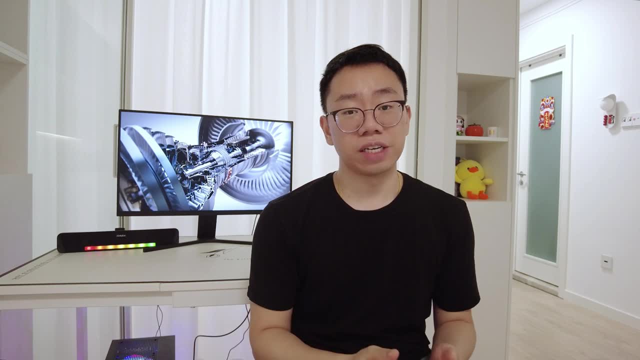 working at big tech companies like Apple, Meta, Amazon and Google, You can climb the corporate ladder to become a manager, director, vice president and potentially the CEO or CTO. The great thing about an engineering degree is that the possibilities are endless. You can. 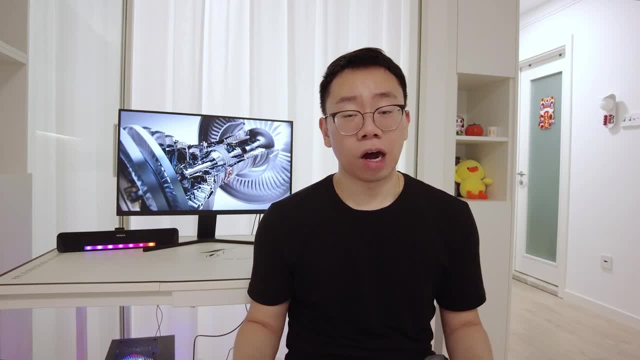 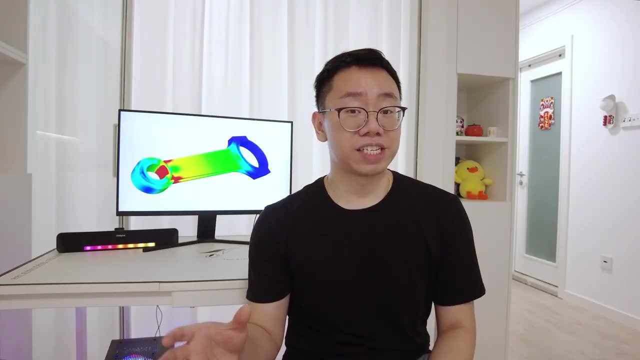 leverage your engineering skill, set and mind to start a business and offer a service or product that tackles a global challenge such as climate change or water contamination. If you succeed, chances are you'll be pretty wealthy, Moving on. not everything you learn in school will be used. 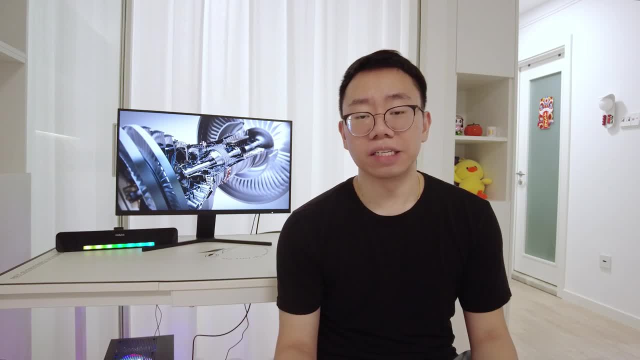 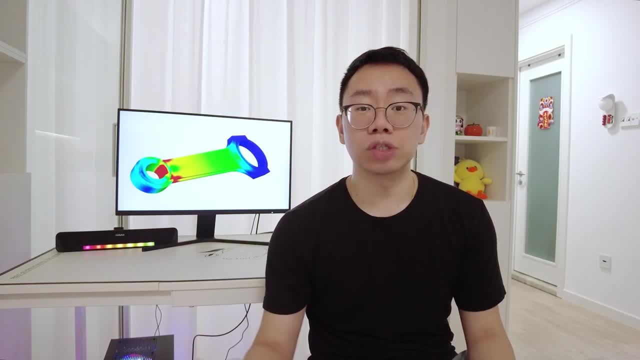 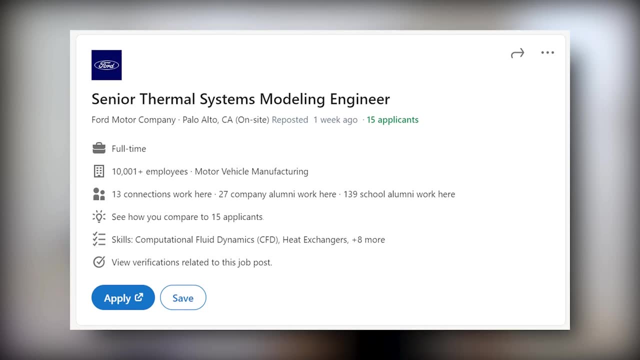 differential equations and thermodynamics class will really be used on the job. Of course, this does depend on which industry you work in and your specific role. For example, if you are a thermal systems modeling engineer at Ford, you will work on improving the performance of HVAC. 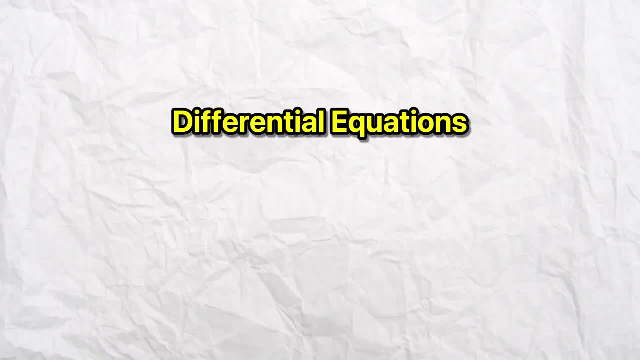 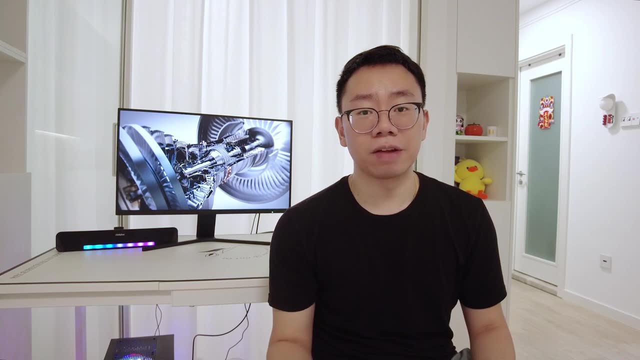 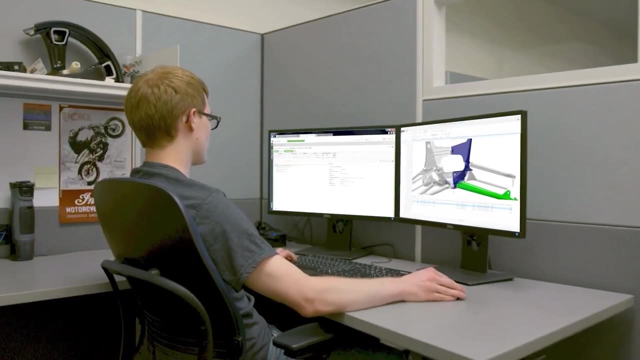 systems in various car models, leveraging knowledge spanning differential equations, thermodynamics, heat transfer and fluid dynamics, and probably use less knowledge from your design and manufacturing. as well as mechanics and materials courses, You'll definitely get a lot of practical knowledge at your first job or internship, such as new design and manufacturing. 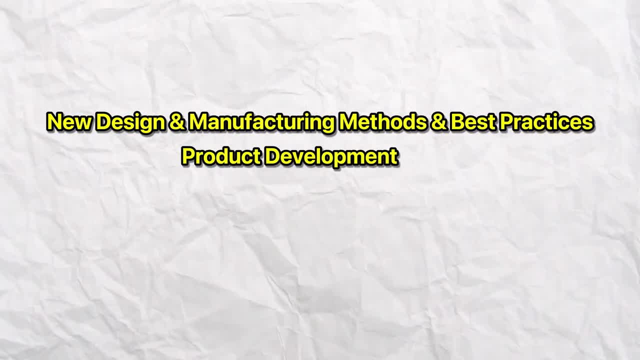 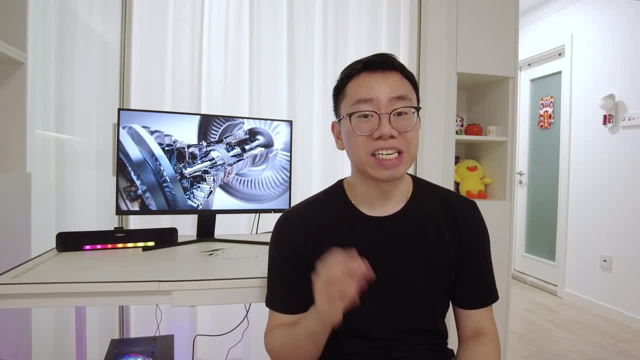 methods and best practices, what the product development cycle entails, how projects are managed and how to work across cross-functional teams. I want to stress that just because a certain class may not be useful in your career doesn't mean you shouldn't try your best in that. 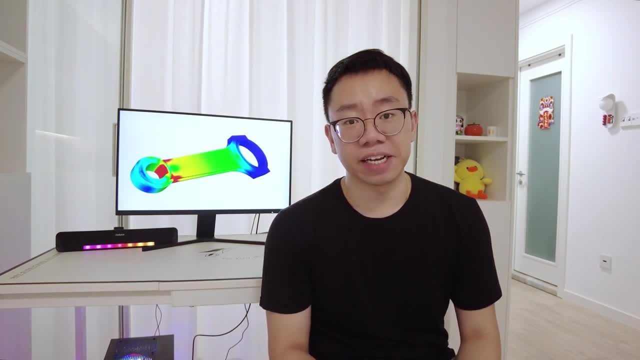 class. Now. I'm not talking about your social science or humanities electives. You can BS your way through those if you want. I'm referring to all of your STEM and English electives. If you want to learn more about STEM and English electives, you can check out my course on my website. 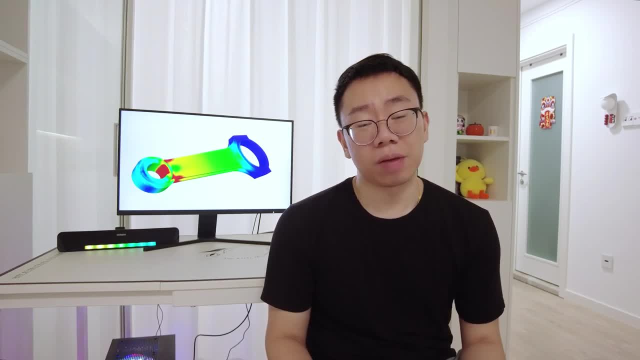 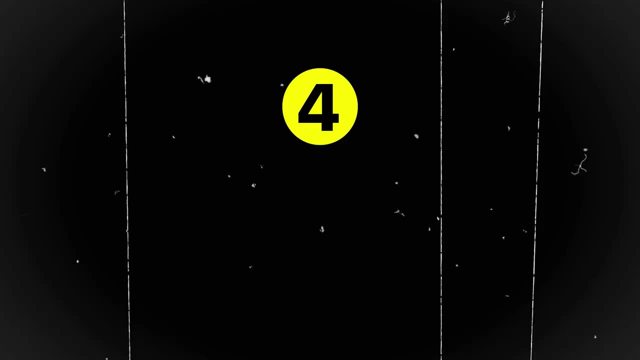 at the link in the description. You never know when the knowledge from that course might come in handy or when you'll need a recommendation or reference letter from your professors for a job or grad school application. On the subject of recommendation and reference letters: networking with people in. 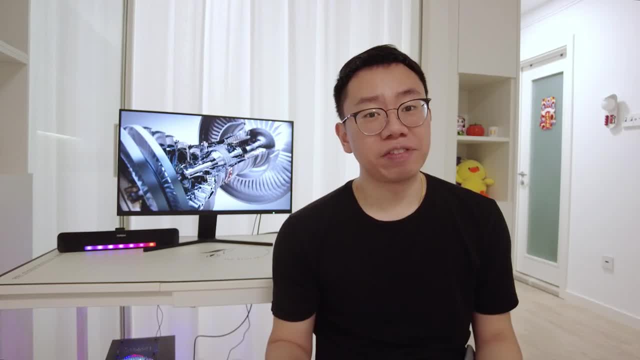 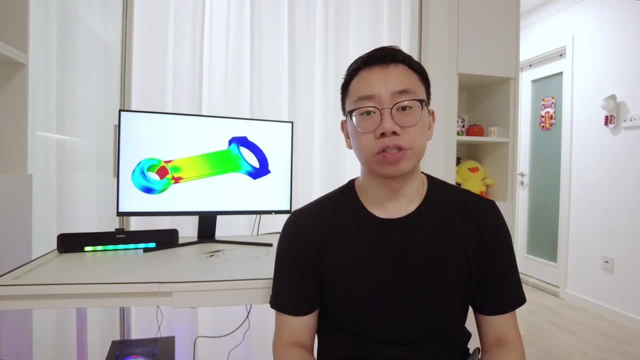 university is absolutely critical. It will inevitably open many doors for you in ways unimaginable. University is the best and last chance for you to make new friends before stepping foot in the real world. so get to know your classmates and professors If you're a student. 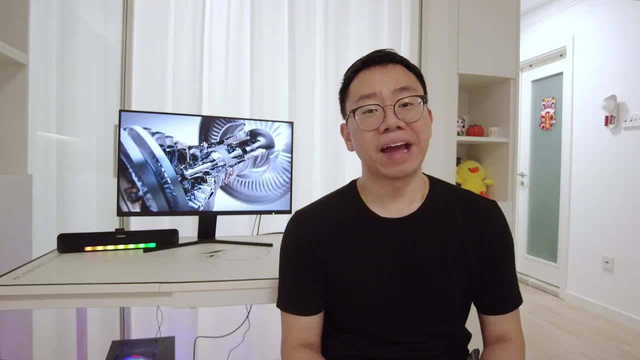 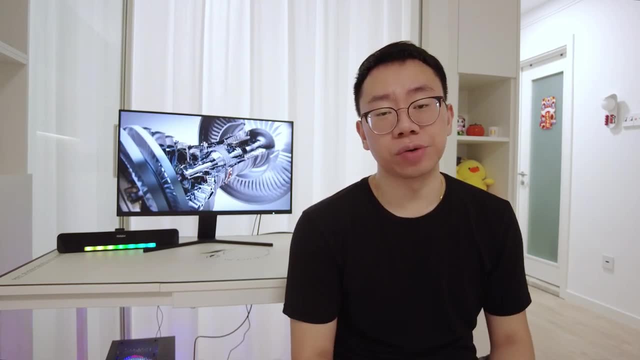 or professor in class, attend career fairs, join clubs and party it up. If you're single, you might even find your soulmate. You'll, without question, have a huge workload as a student, but you still need to find time to socialize. Even though I met all of my best friends in university, I honestly 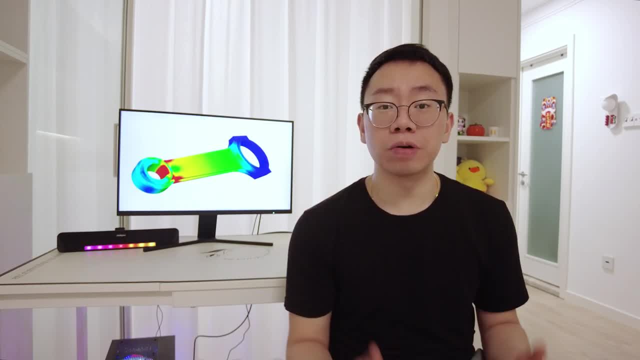 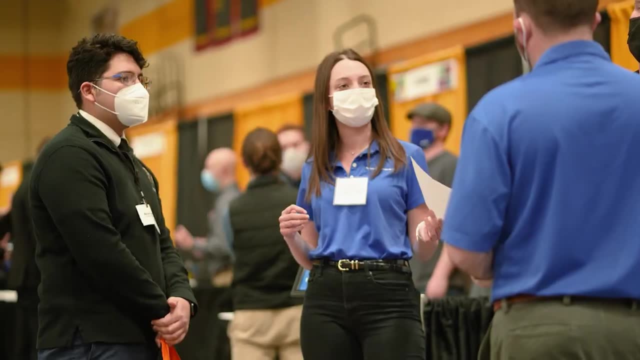 wish I studied less and used that extra time to build more meaningful relationships. Networking is mostly just a numbers game. The more you put yourself out there and meet new people, the higher the chance you'll meet someone who might help you get a job or internship later on. 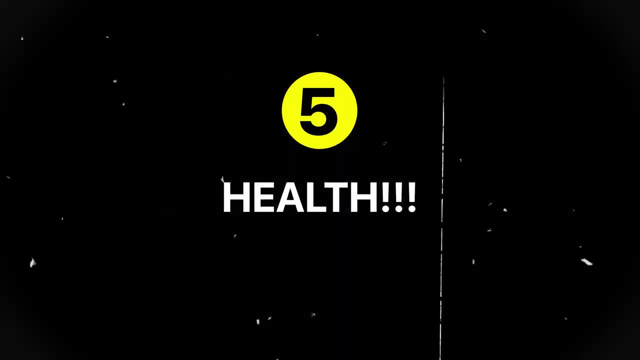 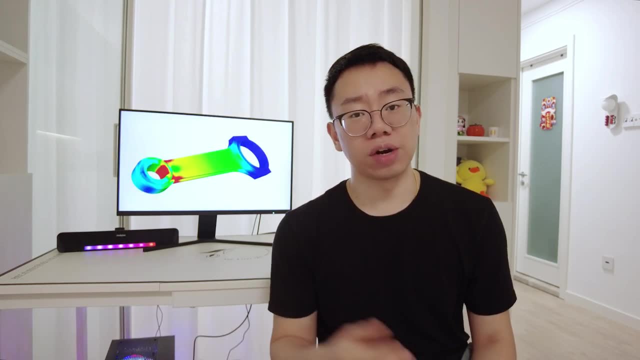 None of the things that I mentioned so far matter without having good health. Your health is your number one priority and trumps everything, including grades, jobs and parties. You need to develop a daily regimen where you eat and workout on time, starting the first day of 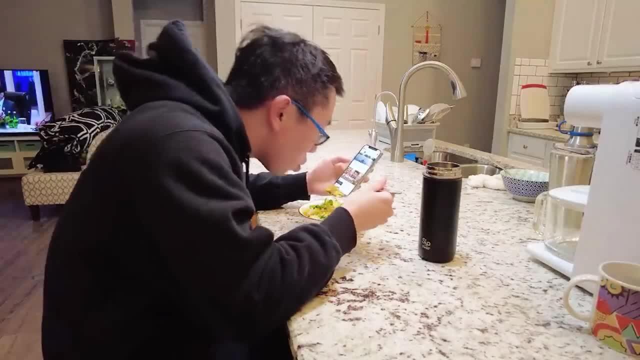 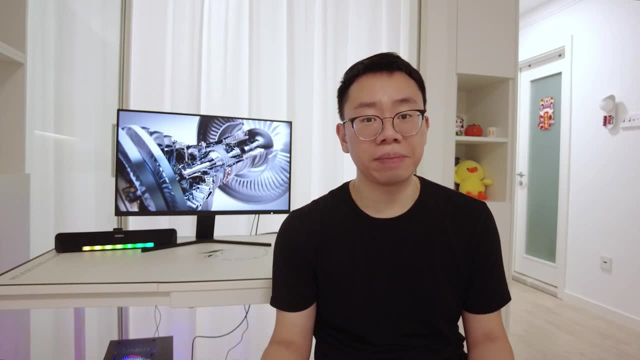 university, Depending on your class schedule, you need to eat at least two or three meals per day and hit the gym at least three times a week. I know how easy it can be to grab a bag of chips for lunch to save time because you're rushing to finish your homework on time. 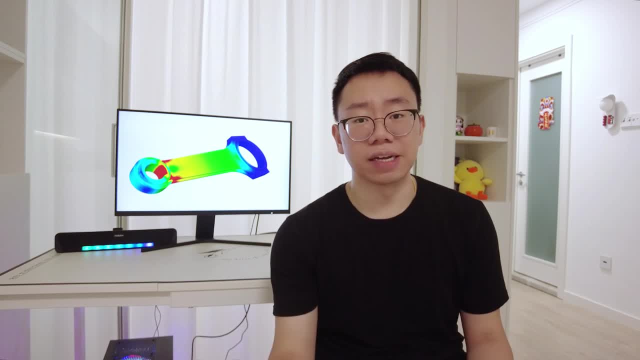 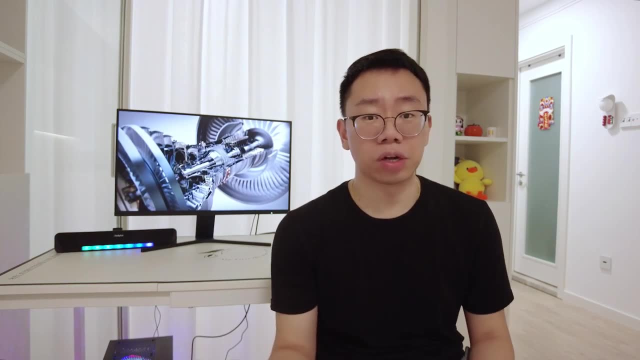 and scrambling to copy answers from Chegg because you procrastinated. Now I'm not saying I did that or anything, but trust me, this is absolutely detrimental to your health in the long run. The six best doctors in life, according to Steve Jobs, are sunlight, rest, exercise, diet. 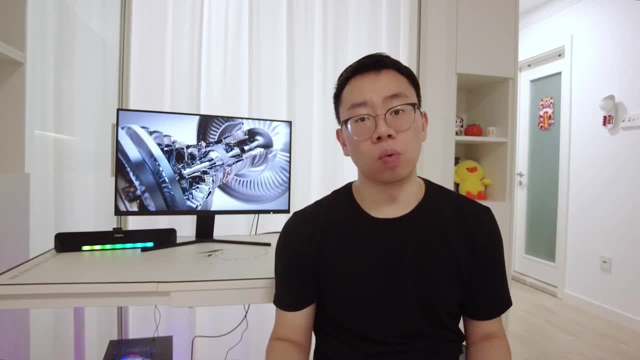 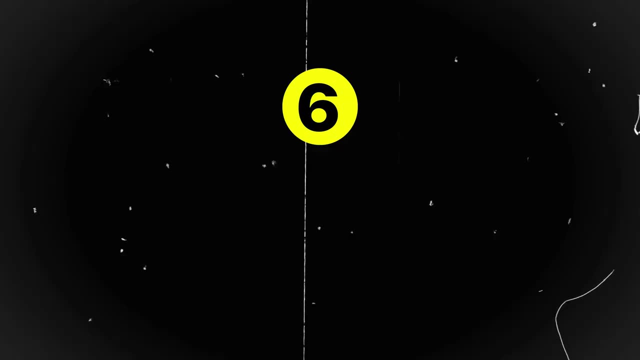 self-confidence and friends, And I couldn't agree more with him. If there's one thing I want you guys to take away from this video, it's this one, This piece of advice. Engineering lectures are notorious for causing students to scratch your 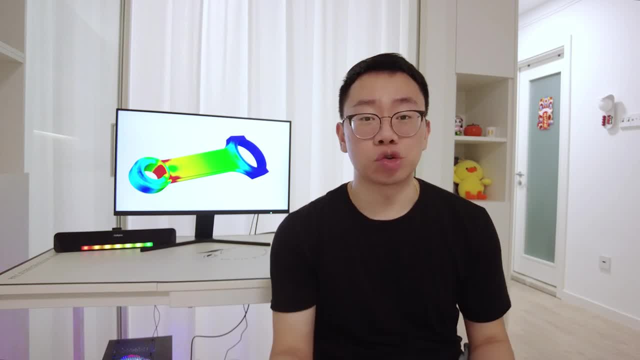 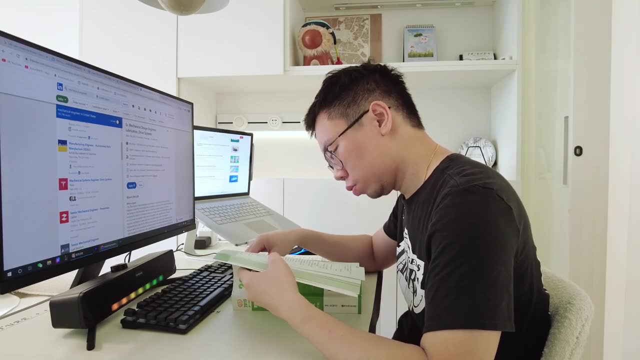 heads because of all the difficult concepts that are taught and the extremely fast pace at which professors teach. Simply take 10 minutes to go over the syllabus and skim through the textbook to familiarize yourself with what's going to be taught in the upcoming lecture. 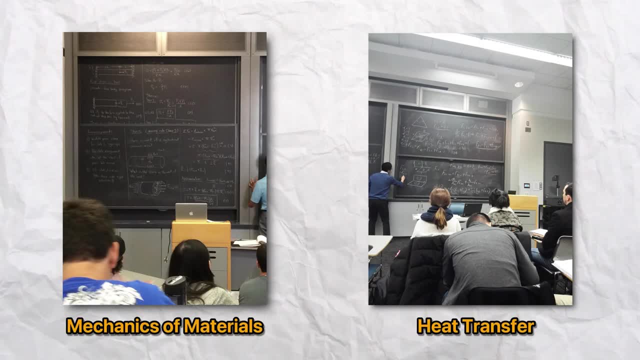 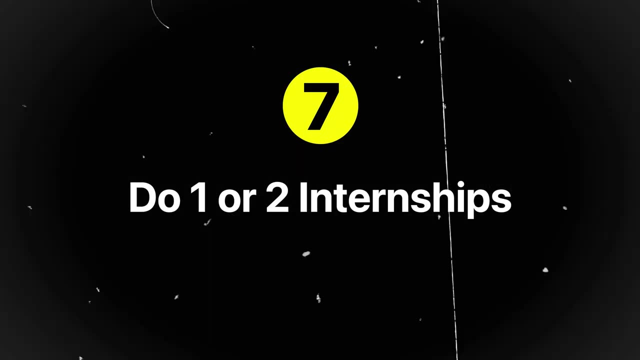 If you're bad at taking notes, get an audio recorder or take pictures of the blackboard and then review the material right after class. Doing one or two internships is a must before you graduate. Nobody will remind or force you to apply to internships, so you definitely need to. 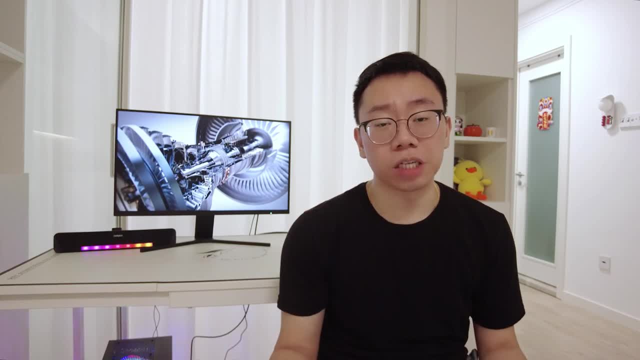 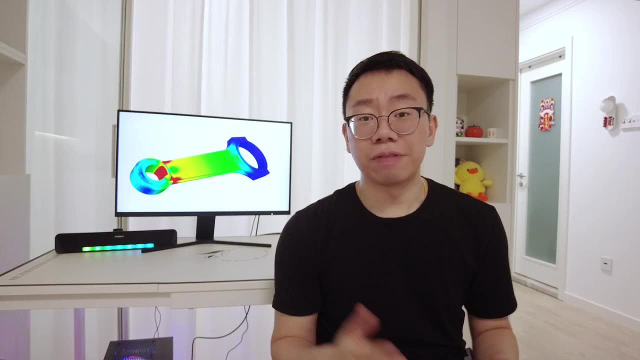 be disciplined. You should start applying as early on as possible, usually starting the spring semester of your freshman year or, at the latest, the spring semester of your sophomore year. Every summer and even winter break that you have should be spent doing internships. 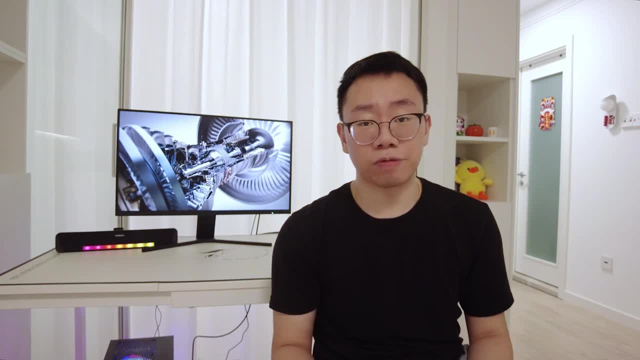 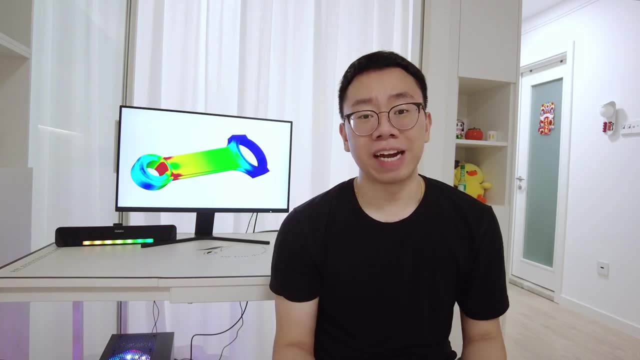 You can find internships through your school's career fair, LinkedIn, friends and family or, if you're interested in a particular company, you can apply directly on their website. If you have trouble finding an internship, reach out to professors in your department or 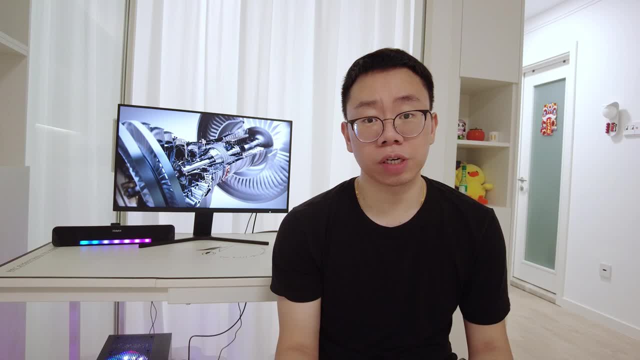 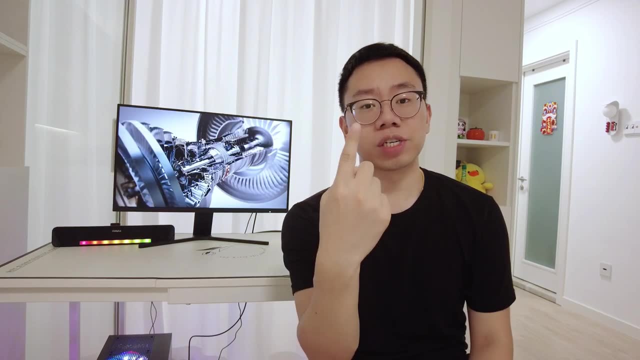 engineering student design teams, such as Robotics or Rocket Propulsion Club, to see if there are any opportunities available. There are two reasons why internships are so important. The first reason is: an internship is the key to landing more job interviews and offers for full-time engineering. 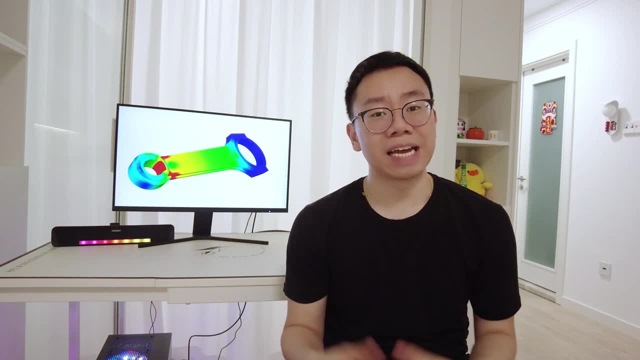 positions once you're a senior. Employers prefer someone who has industry experience and someone who can bring value to their organization. If the company you're working for is a good fit for you, they might even extend an offer for a full-time position. The second reason is a huge chunk of 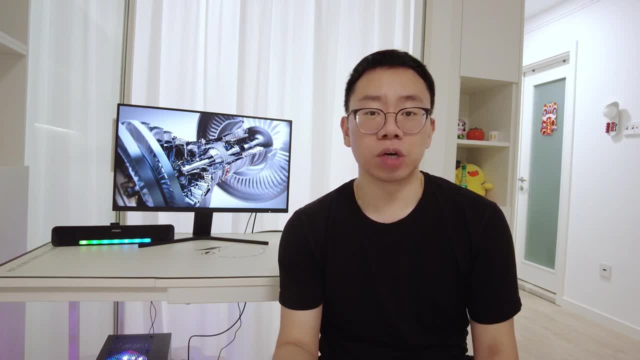 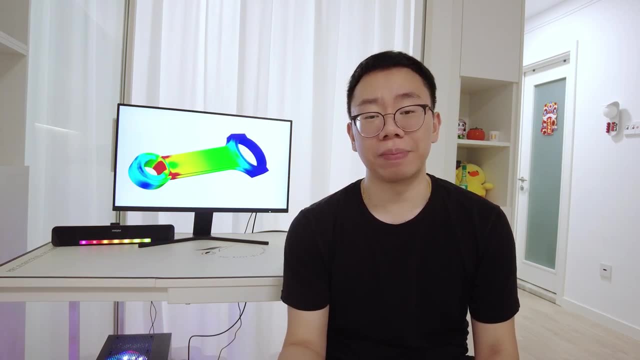 what you learn in school just isn't very practical. so internships equip you with the necessary technical and people skills needed to give you a head start at your first ever full-time job as an engineer. Like internships, you will need to start applying for full-time job opportunities in the 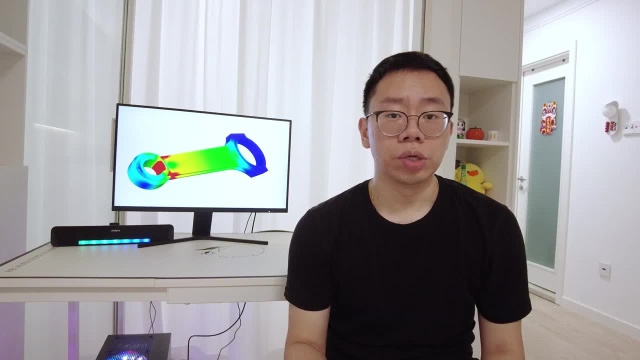 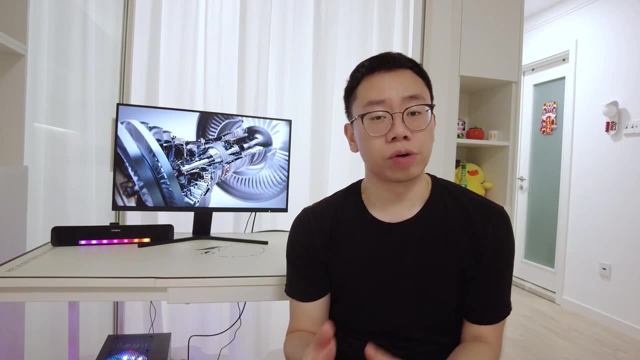 fall semester of your senior year if you don't plan on going to grad school. You want to give yourself sufficient time to land a job, but you're not going to be able to do that in the first place. Go to your school's career fair, as well as their mock interview and resume critique sessions. It's 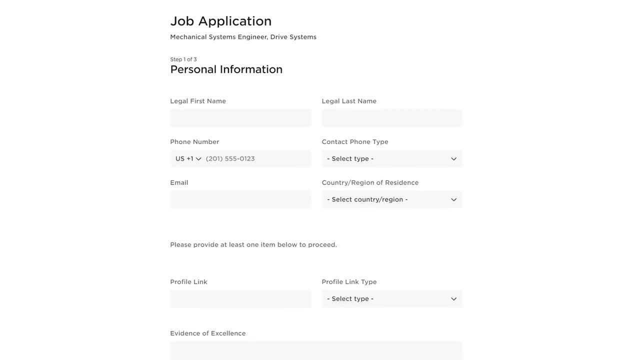 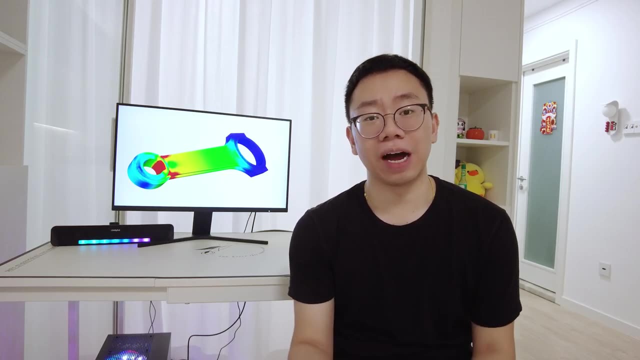 important to apply to as many jobs as possible. So, for example, your weekly goal could be to apply to 30 jobs minimum. Even if you do land a job interview, keep applying. Based on my experience, a lot of things have to go right to get a job offer When you start to get interviews. 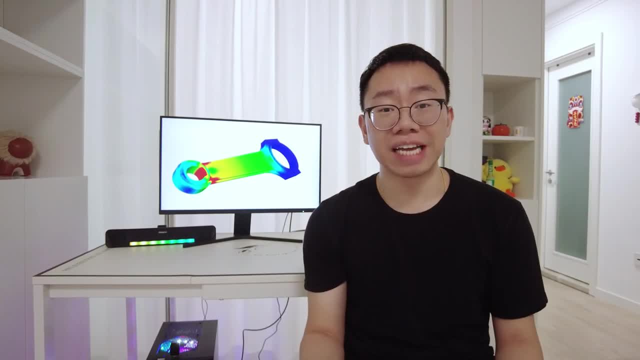 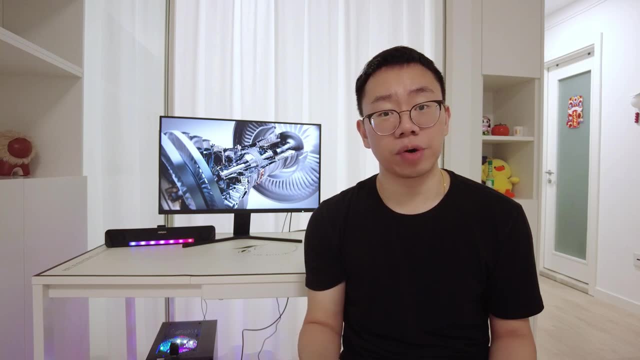 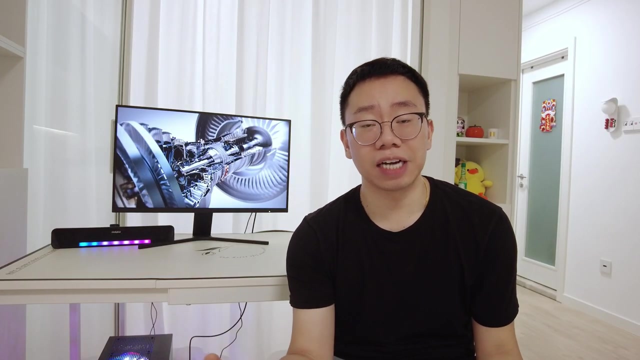 you need to prepare for them. I've interviewed for close to a hundred engineering job positions and the most challenging thing about mechanical engineering technical interviews is you never know what the interviewer, who could be an engineer, engineering manager or panel of engineers, will ask. This is one of the biggest roadblocks that I see many fresh mechanical 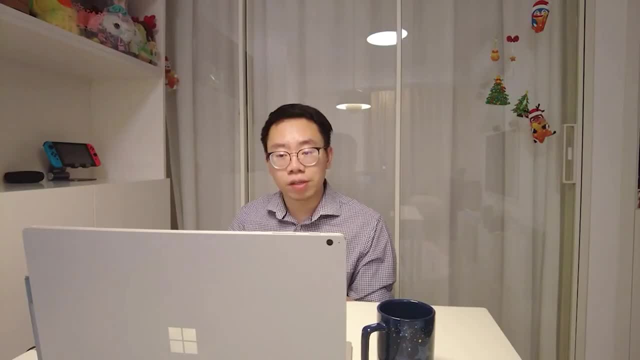 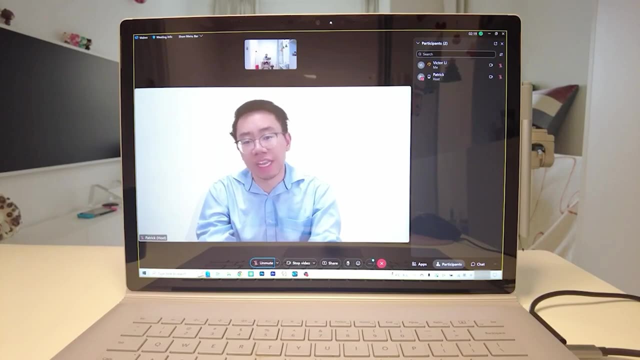 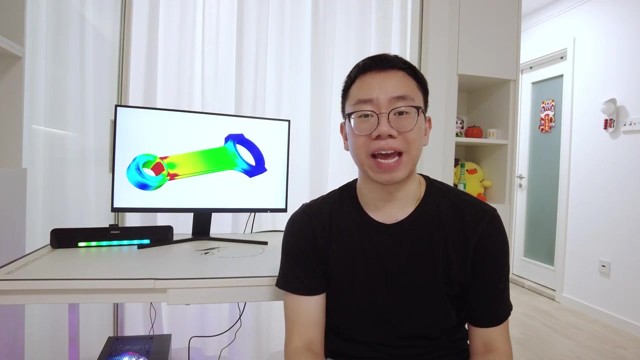 engineering graduates, including my former self, struggle to overcome because the questions that employers ask are either very specific or have to do with technical challenges that they're currently facing. To help you guys out, I put together a list of 80 technical questions spanning all areas of mechanical engineering that I think are great. 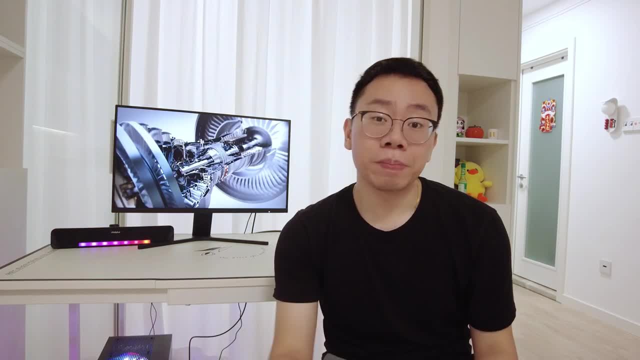 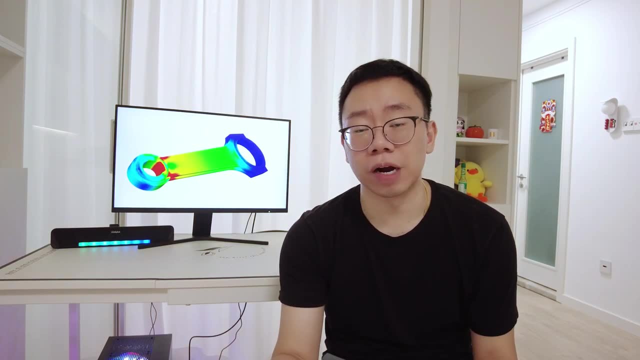 to know and hopefully will help you land your dream job. Keep in mind that the solutions are not included. I think it's very beneficial to think through problems yourself, which helps you better prepare for technical interviews instead of memorizing answers and regurgitating. 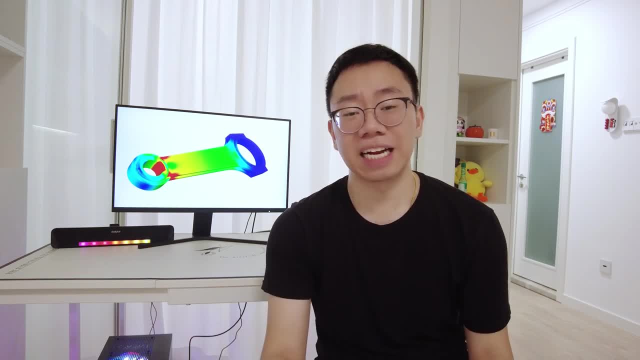 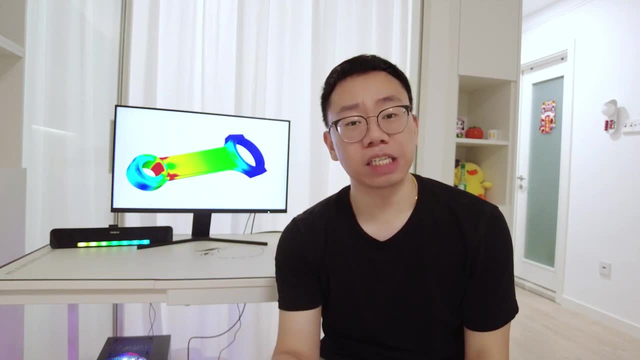 them in an interview. So if you're interested, be sure to check out the link in the description below. When you're applying to jobs, keep in mind that every engineering job is different. Ask what aspect of engineering excites you the most and what type of company you want to work for. Some 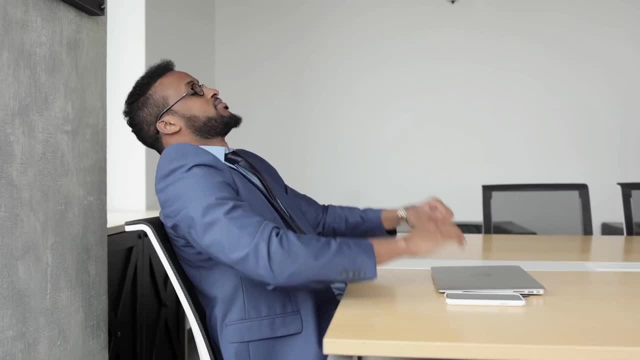 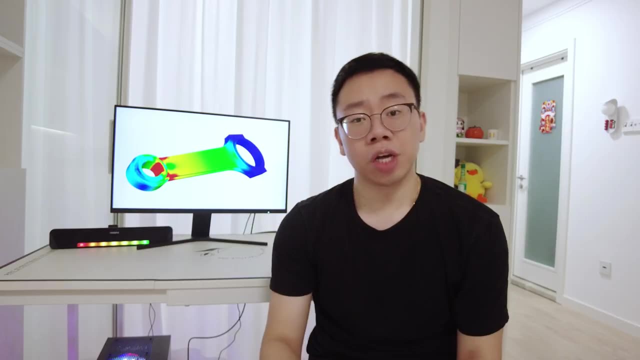 jobs are actually quite depressing and crack the whip pretty hard, so you're always left feeling burnt out, while other jobs are the polar opposite, where you sit around all day bored out of your mind. Some red flags to look out for in a job description include: can multitask, fast-paced. 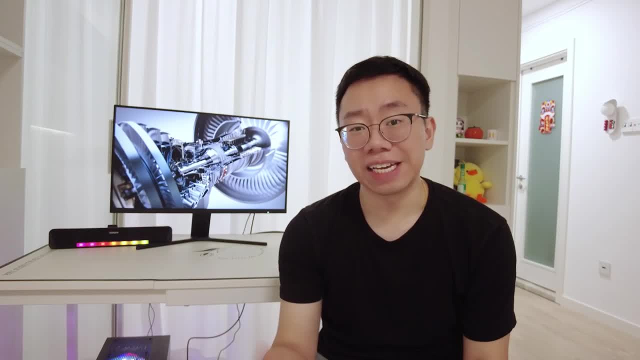 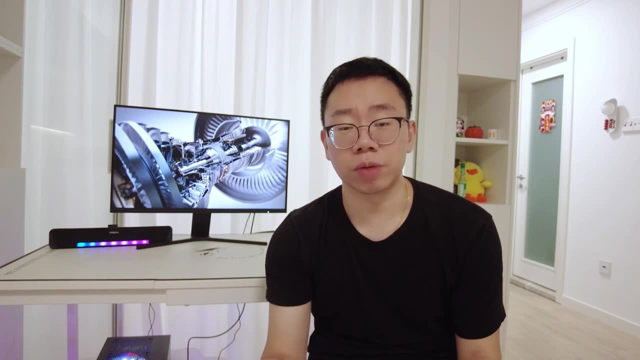 environment must be able to work under pressure. It could be a sign that the work environment is toxic, but not necessarily. Generally, startups require long hours and commitment from their workers to get them off the ground. It's likely you'll wear multiple hats and work on different projects in parallel at a startup. 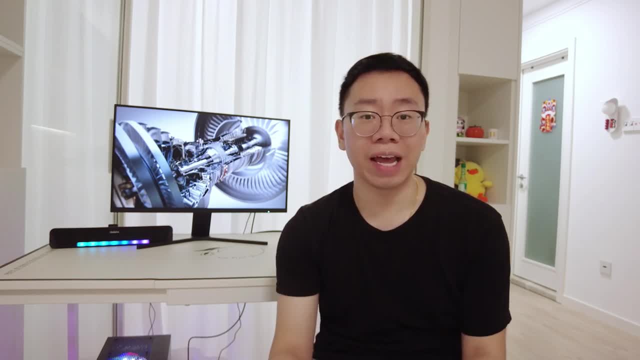 On the other hand, larger companies like General Electric or Boeing might have you work on a very specific part of a product. So if you're working at Airbus, you wouldn't be responsible for designing the entire aircraft, but instead, say, a sub-assembly of the plane's rudder. 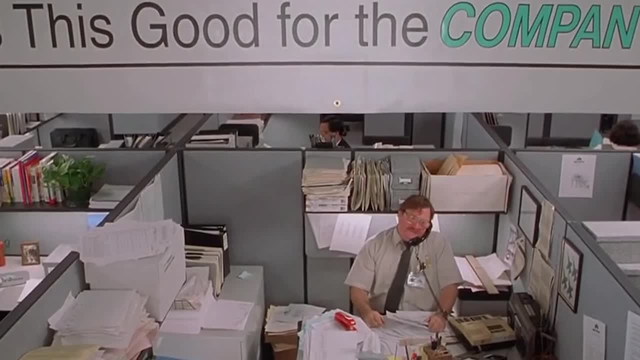 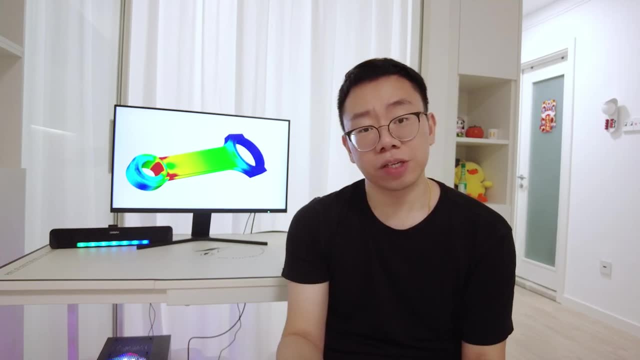 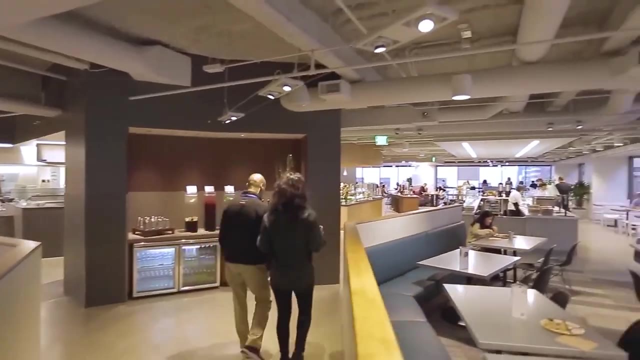 Companies with a toxic culture will probably have you working in a poorly lit office with cubicles like this, with very little human interaction and a dirty cafeteria, While companies with a positive culture will have a contemporary open office format with large windows and a cafeteria that looks like a restaurant. Some examples include Apple, Google, Amazon. 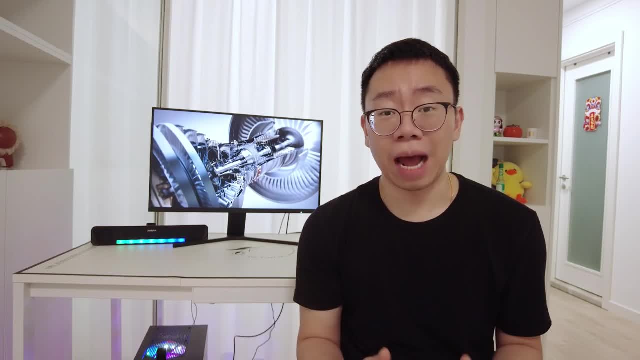 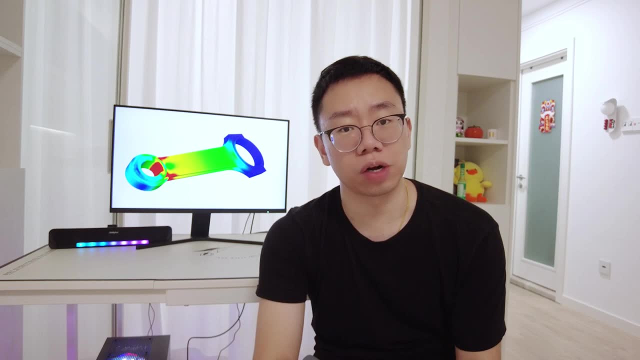 Meta and LinkedIn. You know you've found the right job when you feel happy, empowered and motivated to get up in the morning for work. Ask yourself which industry and products you would like to work on. Maybe you want to design the next generation. 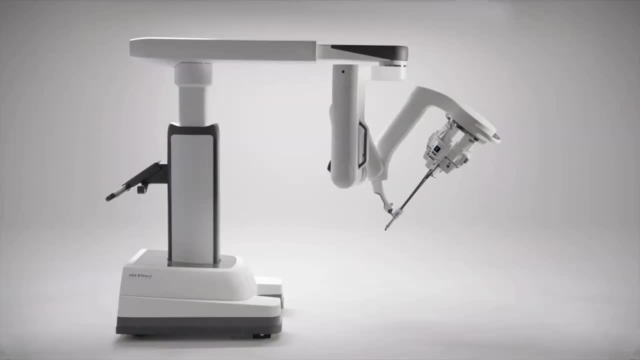 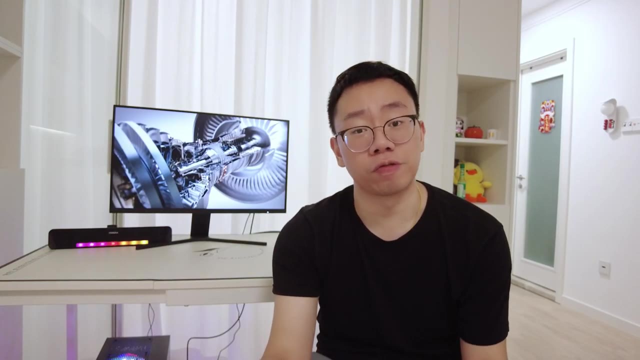 of Apple iPhone in the consumer electronics industry or the cutting-edge intuitive DaVinci surgical robot in the medical industry. It's totally okay if you can't get into these companies for your first full-time job, but try to look for opportunities within the same industry. 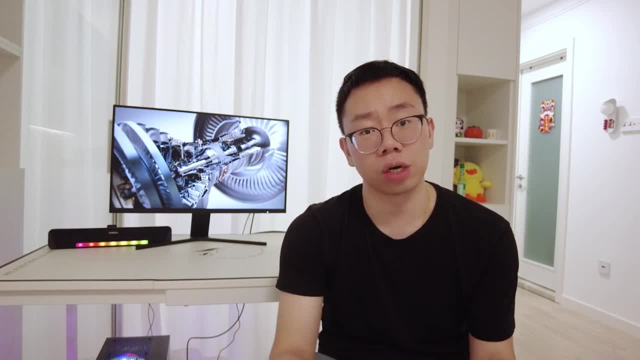 so it's easier for you to make the transition in the future. People who don't truly understand engineering just think that we just design and build cool stuff, But the reality is virtually every engineering job, whether it involves designing phones, airplanes, cars, etc. will be designed and built in the future. So if you're looking for a job, that's. 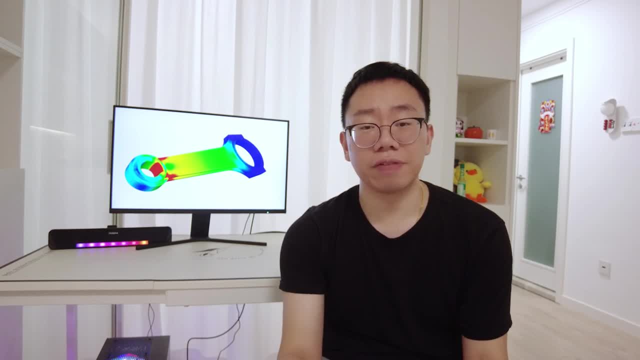 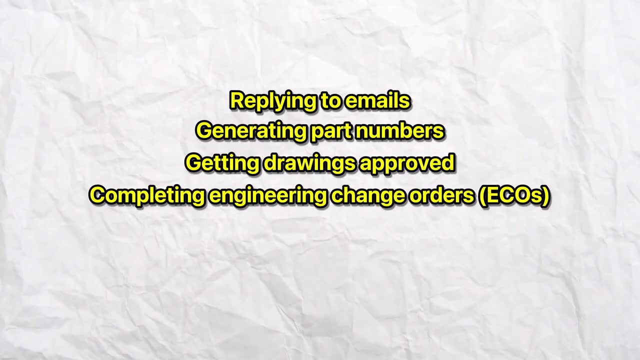 like ours or robots. it involves pushing paper and a lot of administrative tasks like replying to emails, generating part numbers, getting drawings approved, completing engineering change orders, attending meetings and making presentations. Designing the actual parts in CAD prototyping.